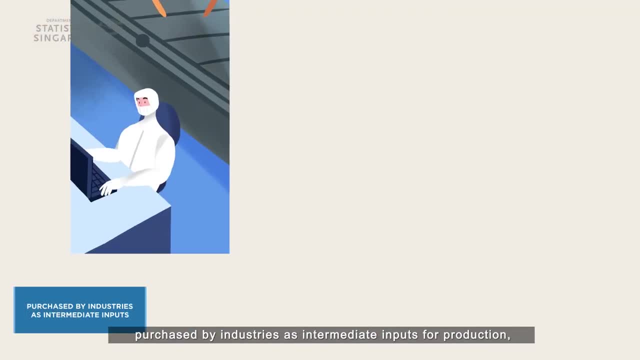 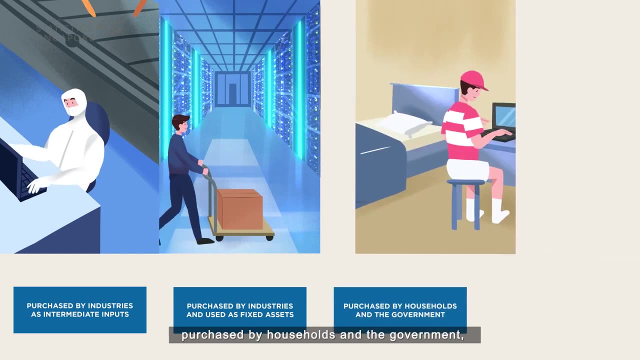 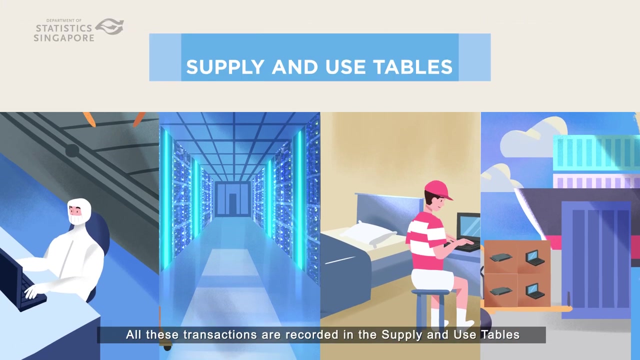 These goods and services can be purchased by industries as intermediate inputs for production, purchased by industries and used as fixed assets, purchased by households and the government, or exported to other countries. All these transactions are recorded in the supply and use tables, which provides answers to three key questions. 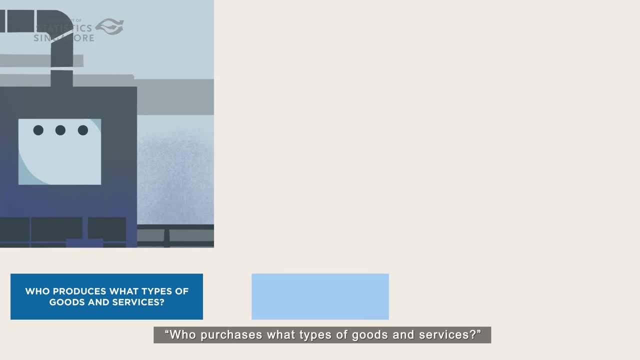 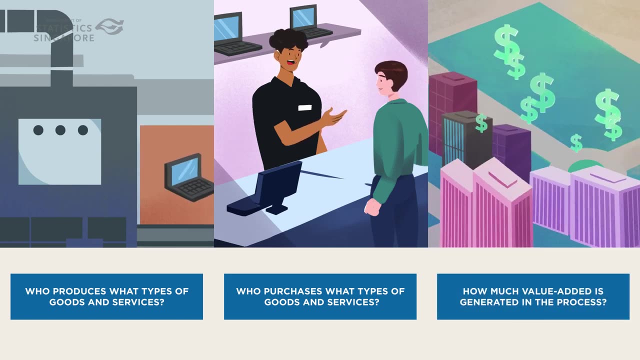 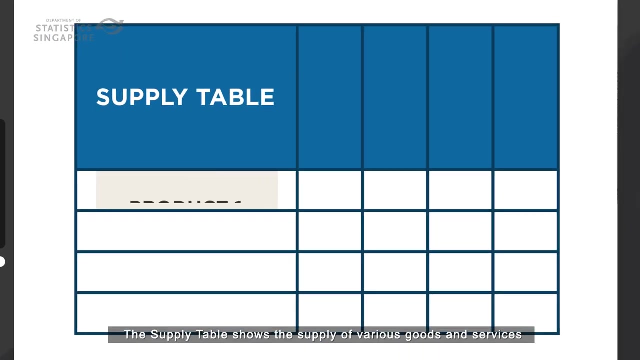 Who produces what types of goods and services, Who purchases what types of goods and services And how much value added is generated in the process. Let's see how these questions are answered using the supply and use tables. The supply table shows the supply of various goods and services. 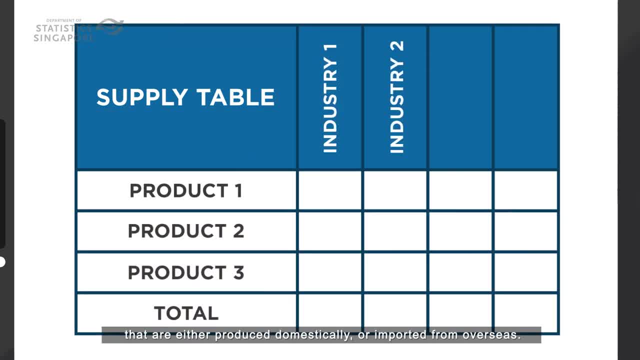 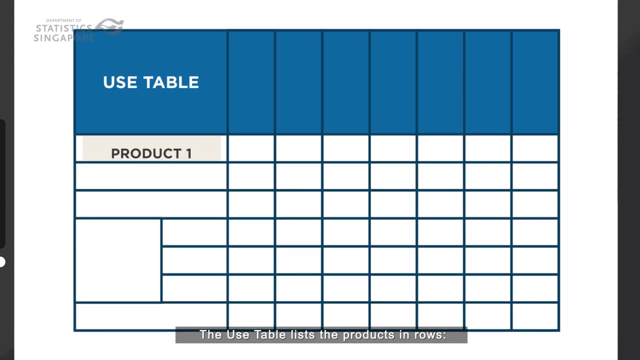 that are either produced domestically or imported from overseas. In other words, it answers the question: who produces what types of goods and services? Products are shown in rows, while the domestic industries and imports are shown in columns. The use table lists the products in rows. 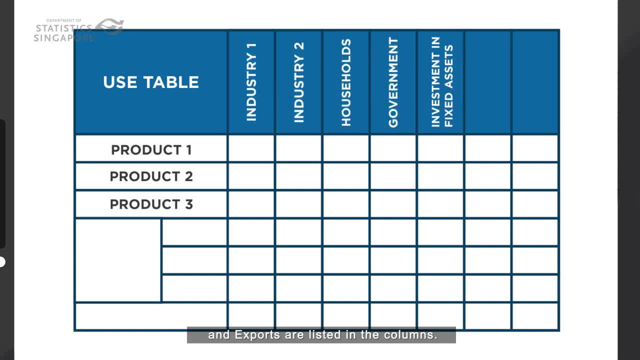 Industries, households, government investment and fixed assets and exports are listed in the column. It answers who purchases what types of goods and services. The use table also shows the value added generated by each industry. Value added consists of wages paid to employees. 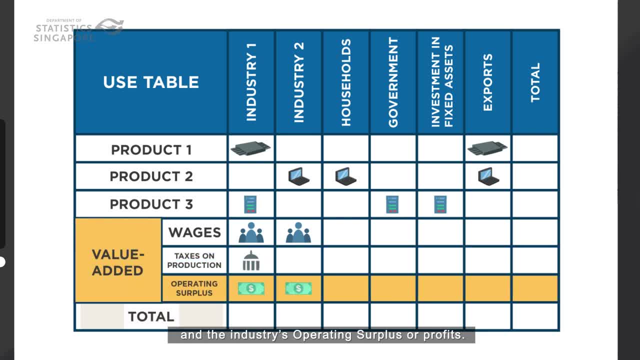 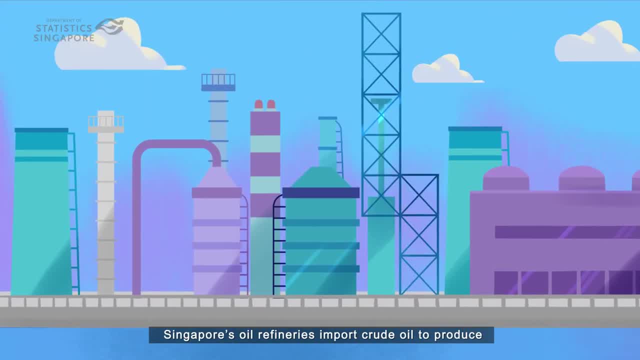 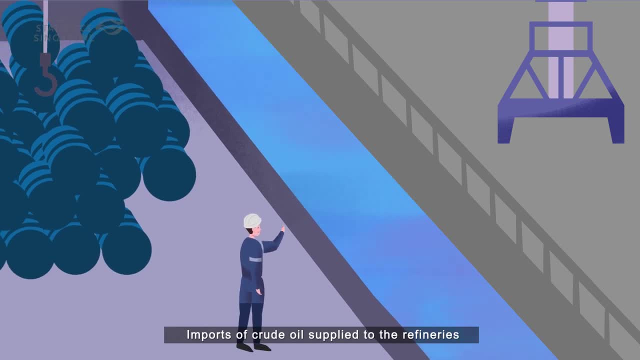 taxes on production and the industry's operating surplus or profits. Using an example, let's see how the various transactions are recorded. Singapore's oil refineries import crude oil to produce refined petroleum products such as jet fuel. Imports of crude oil supplied to the refineries are recorded in the 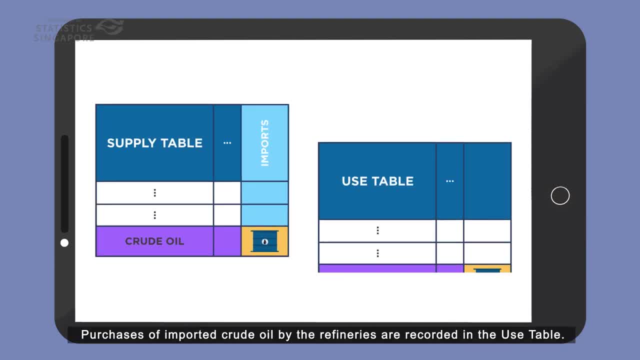 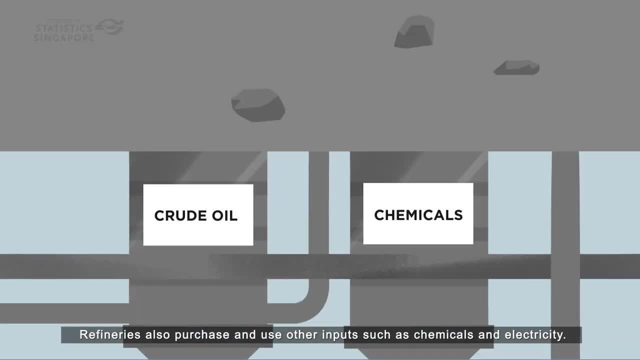 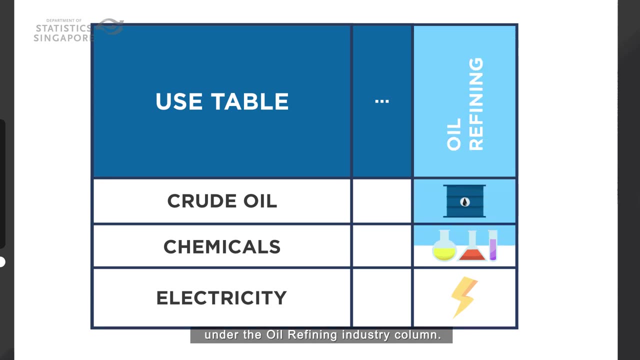 imports column of the supply table. Purchases of imported crude oil by the refineries are recorded in the use table. Refineries also purchase and use other inputs such as chemicals and electricity. These additional inputs are recorded in the use table under the oil refining industry column. 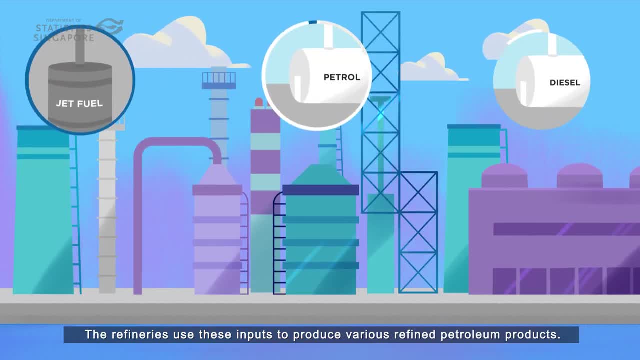 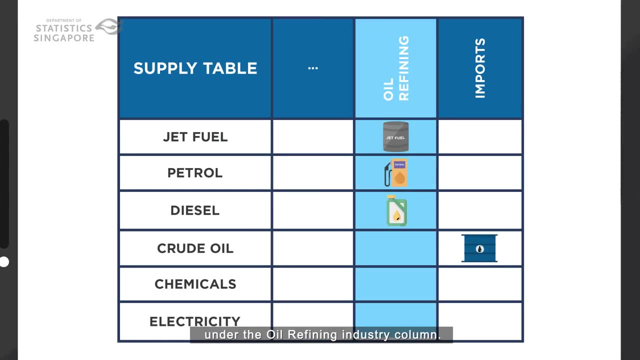 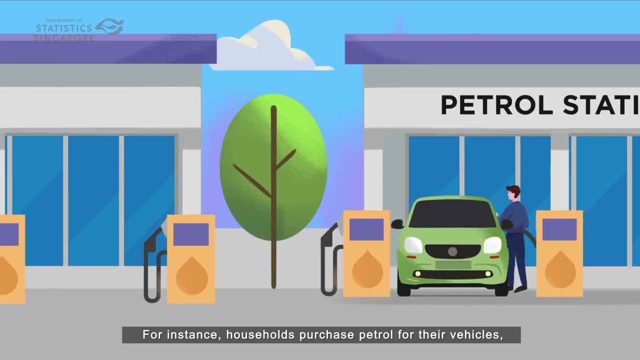 The refineries use these inputs to produce various refined petroleum products. The transactions are recorded in the supply table under the oil refining industry column. These refined petroleum products are supplied to various groups of consumers. For instance, households purchase petrol for their vehicles, airlines purchase jet fuel and diesel is exported to overseas markets.